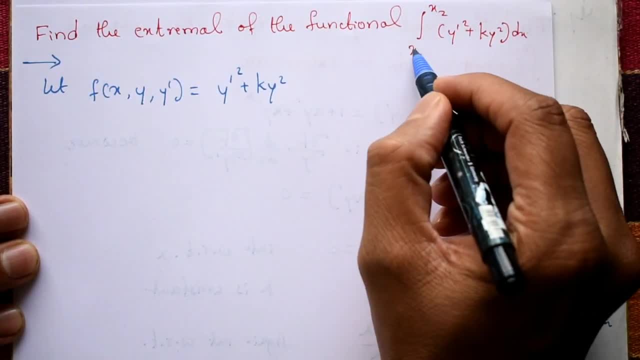 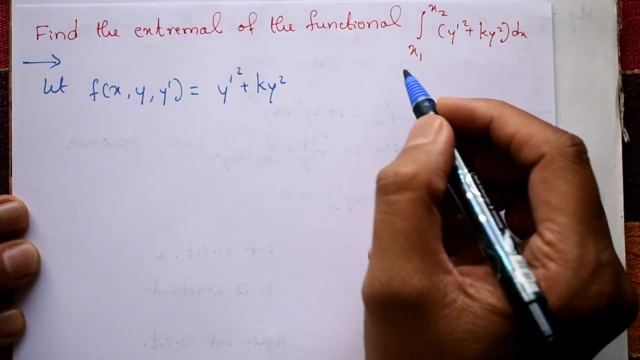 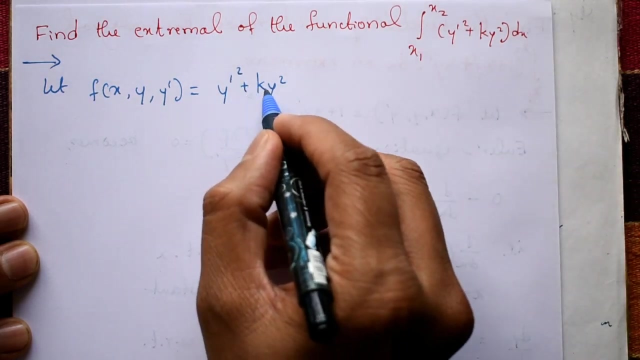 Find the extremal of the function functional integration of x1 to x2: y dash square plus k? y square with respect to x. Okay now solution: This problem is very simple. Let this part you consider, that is f, of x, y, y dash is equal to y dash square plus k? y square. Okay, now we follow the Ehlers equation. 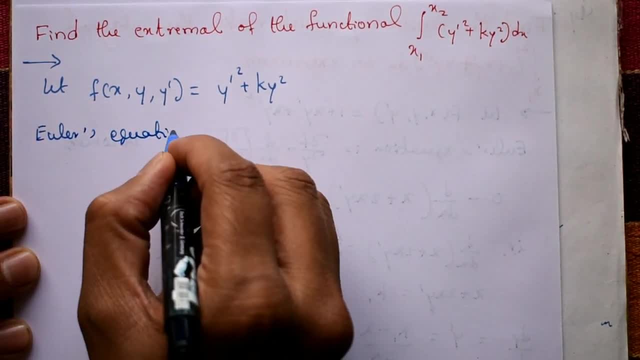 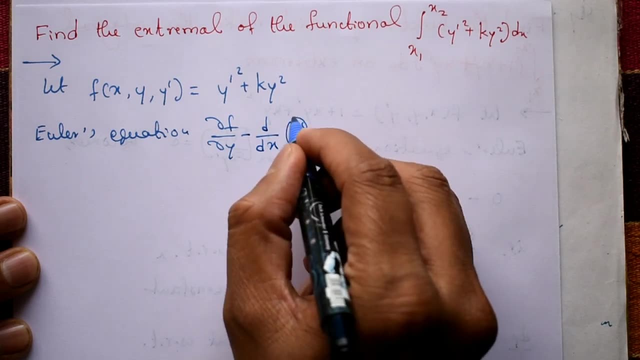 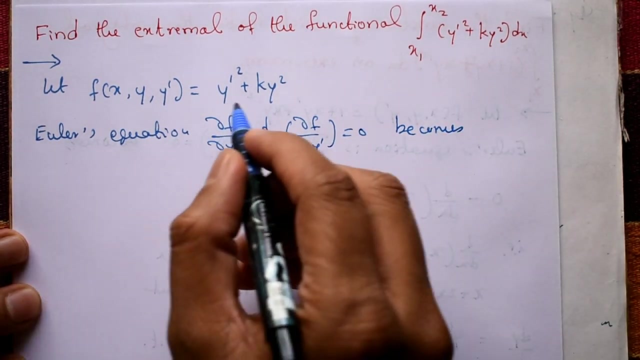 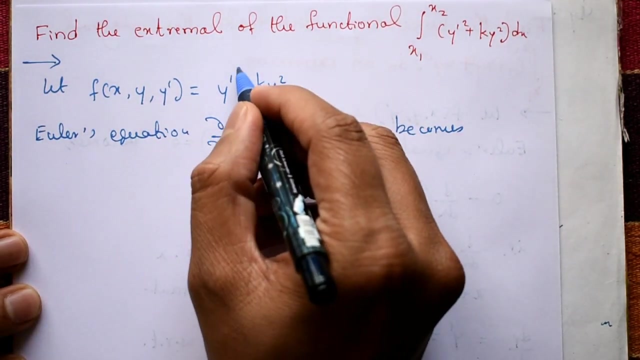 Okay, Ehlers equation is dou f by dou y minus d by dx into dou f by dou y dash, that equal to 0.. This equation becomes Okay. now differentiate this function with respect to y. No y variable. Sorry, k y square is variable. is there y y dash, whole square is 0.. Only we differentiate y. 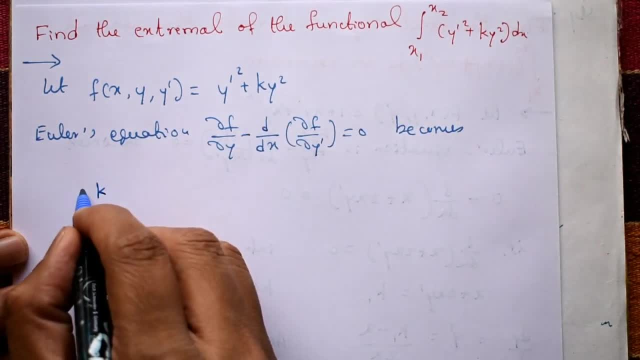 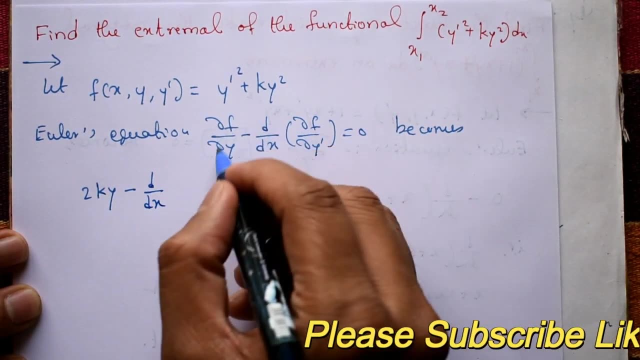 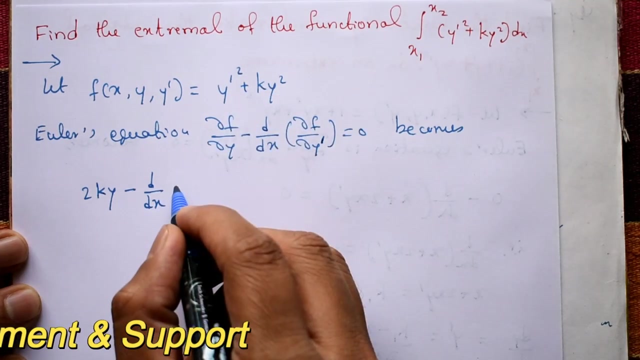 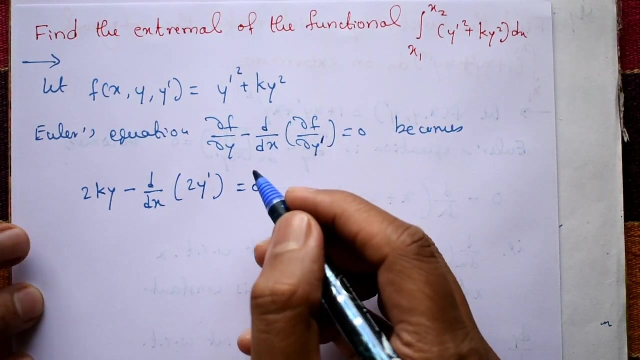 Okay, k is a constant k as it is y square differentiate, you get 2 y 2 k. y minus d by dx. Dou means pd. Differentiate this function with respect to y dash. Other variables are constant. This is 0.. Only y dash differentiate. You get 2 y or 2 y dash. that equal to 0.. Okay, or take 2 divided by 2 means we get 2 y. 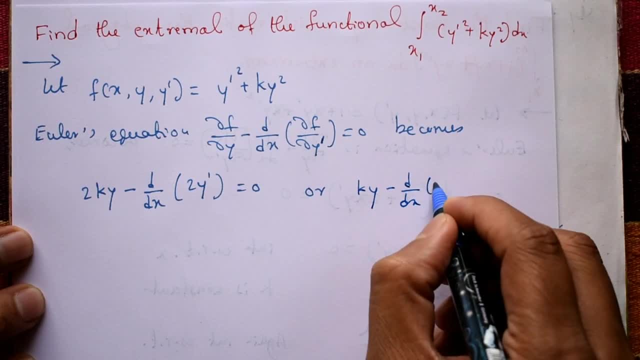 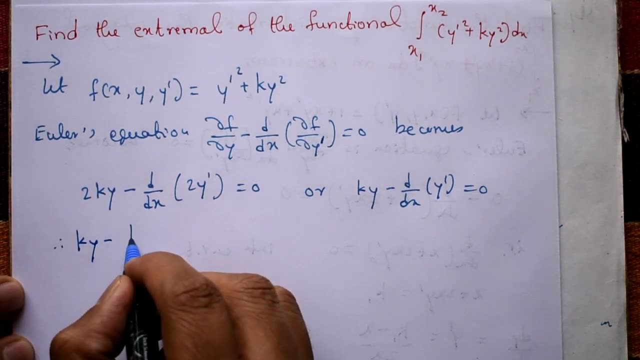 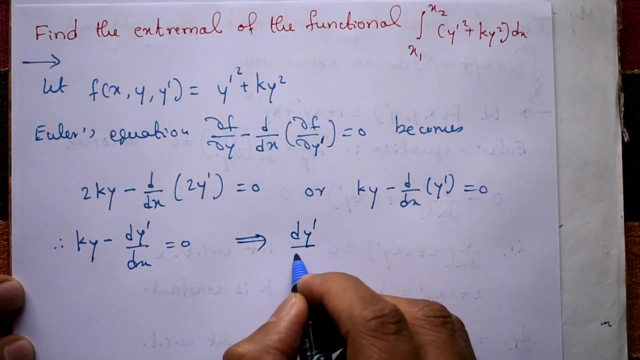 Okay, k y minus d by dx into y dash, that equal to 0. Okay, now therefore, k y minus d y dash by dx, that is equal to 0.. Now change the sign means: d y dash by dx minus k y equal to 0.. Now differentiate y dash with respect to x. Once again differentiate with respect to y dash. we get y double dash. 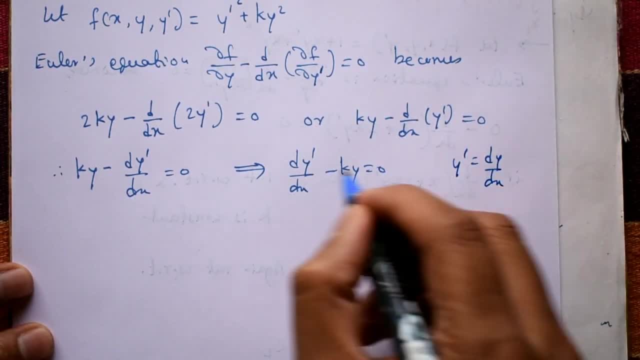 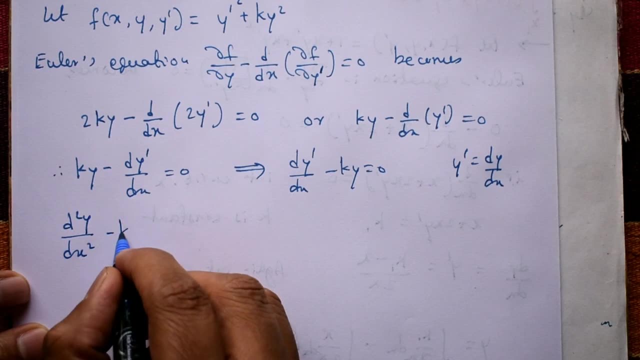 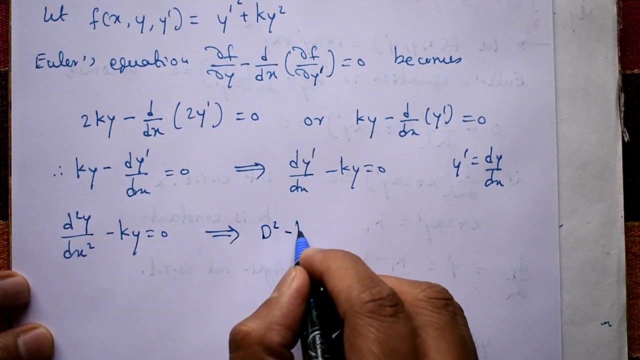 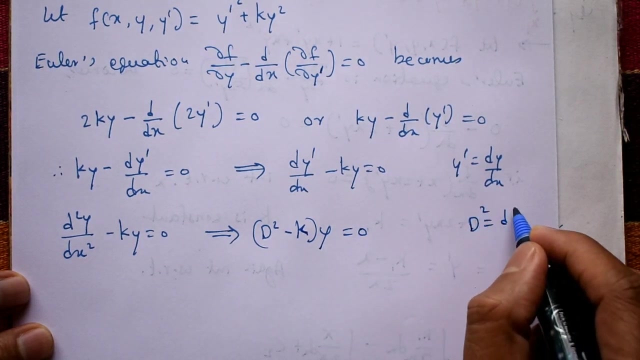 Second order: y dash means what? d y by dx, Again with respect to x, means we get d square, y by dx square, or y double dash minus k, y equal to 0.. Okay, this is equal to d square minus k. into y, Take y, that is equal to 0.. Now d stand d square, stand d square by dx square or d stand d by dx. 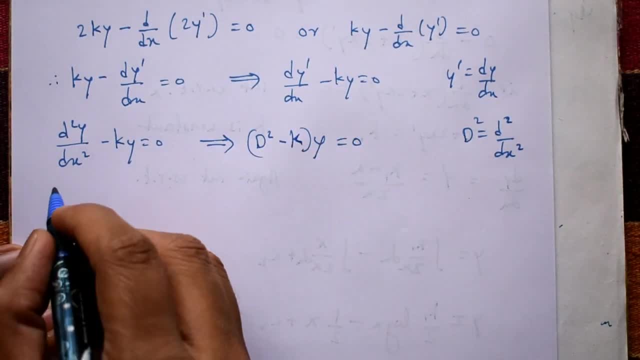 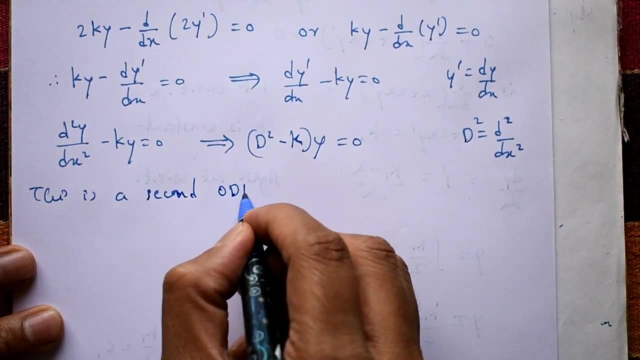 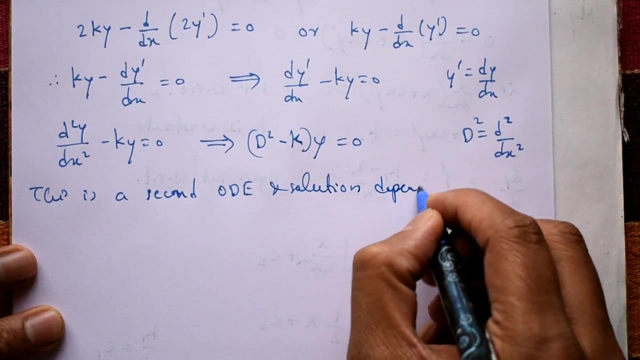 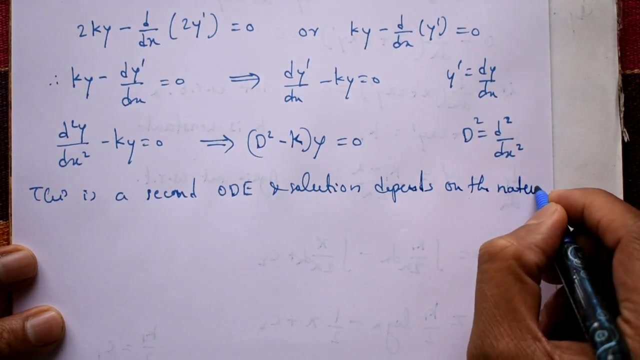 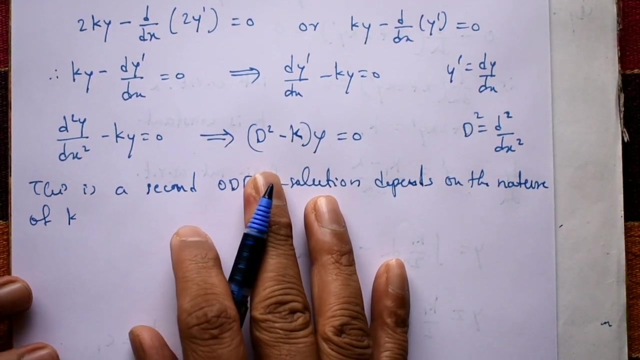 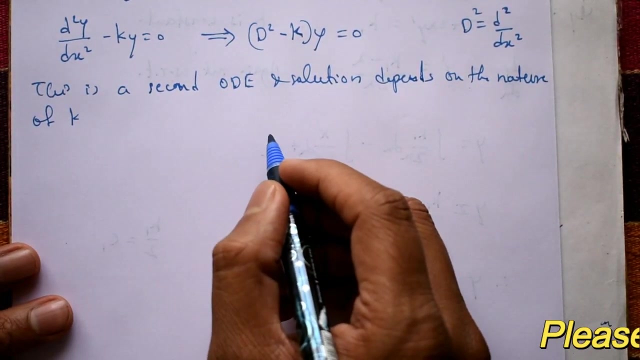 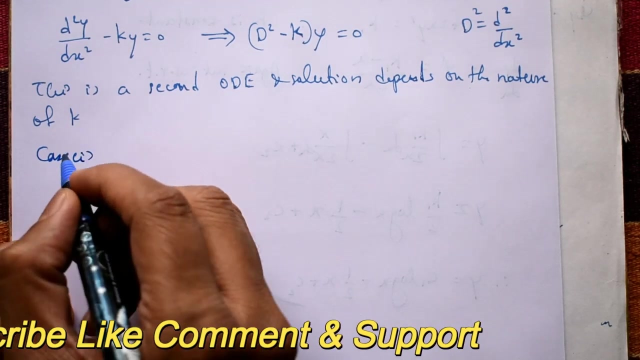 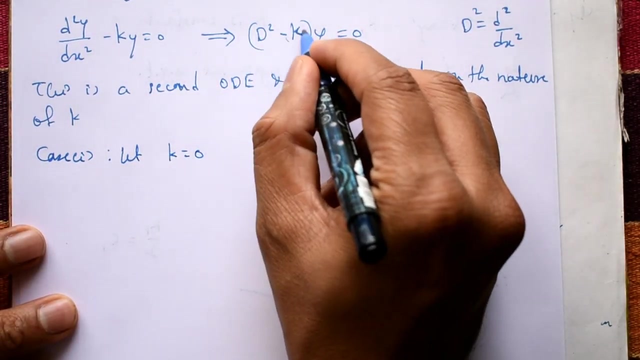 Okay, now see this equation. Now this is: this is a second order, ordinary differential equation and the solution depends on now this solution depends on the nature of the k, nature of the nature of k. So taking on this k value. So taking k value, 1 is positive, 1 is less than 0, 1 is greater than 0, or 1 is k is equal to 0.. 3 possibilities, sorry, 3 possibilities. Now case 1, now take first case. now take k is equal to 0.. Now put k is equal to 0. in this equation we get d square y is equal to 0.. 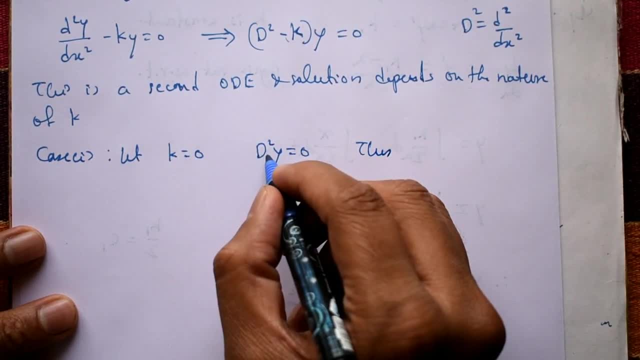 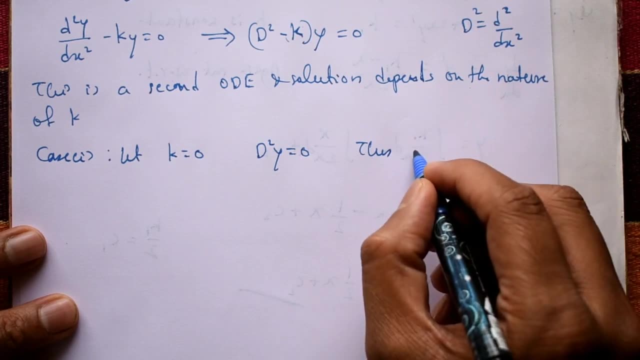 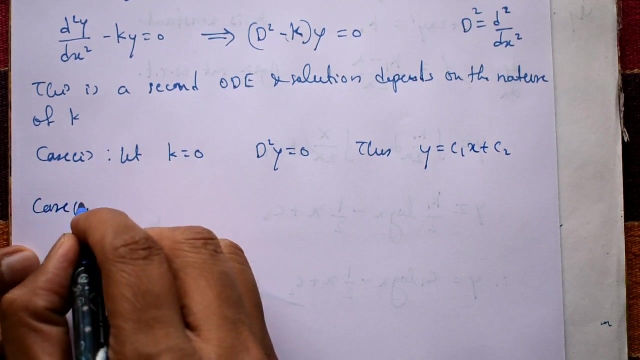 Now. thus: d square means oxygen. equation is: m. square is equal to 0, m is equal to 0, 0. two roots are equal, but roots are 0. that general solution is: y is equal to c1, x plus c2. okay, now case two. 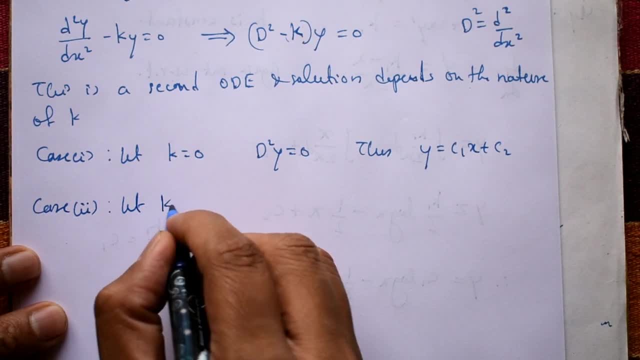 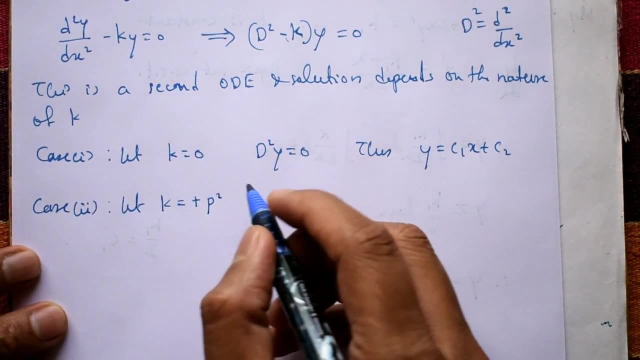 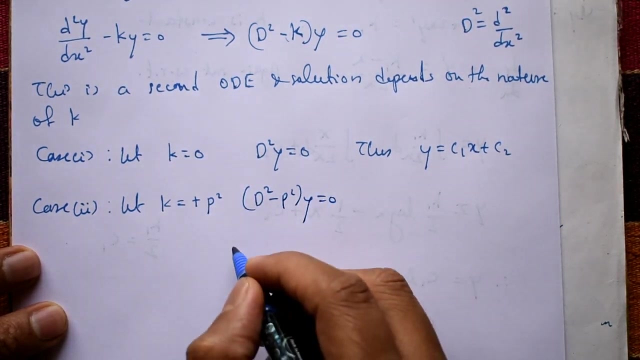 let i'll take positive k value is a positive plus p square. will consider because second order, ode now. take k is a p square. now then k square minus p square into y equal to 0. now auxiliary equation is: d square minus p square is equal to 0, or d square is equal to. 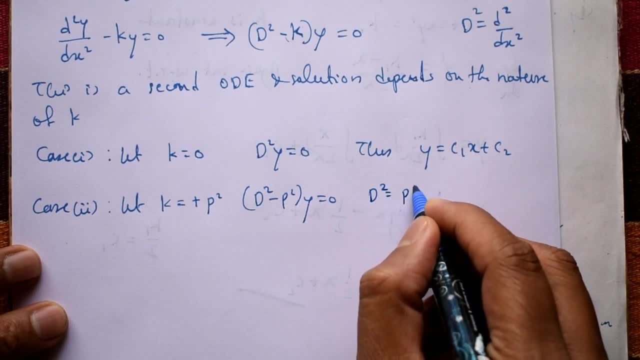 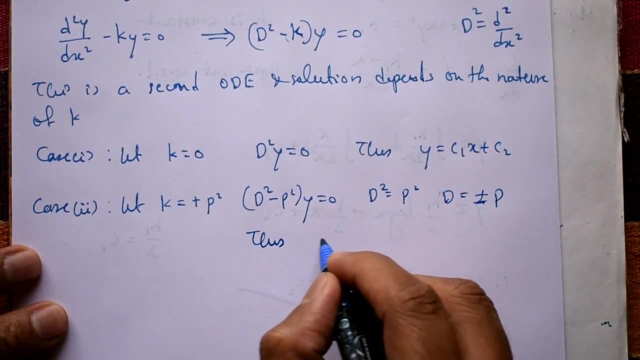 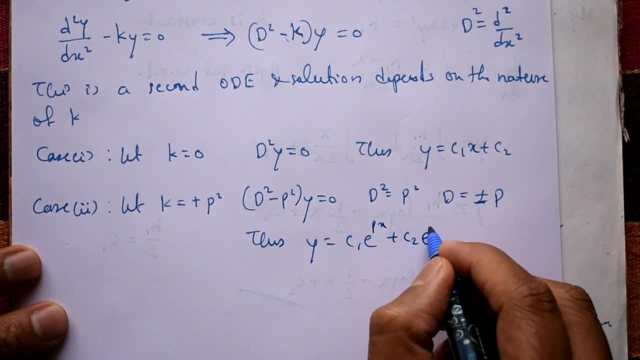 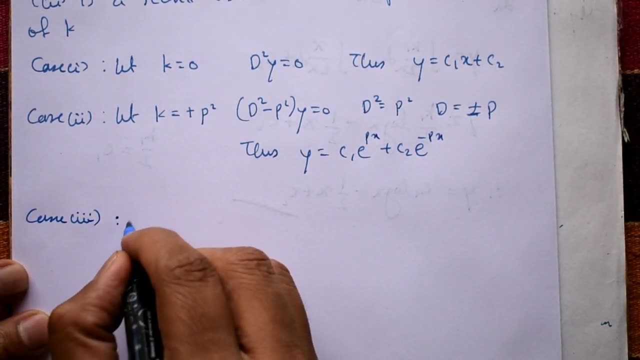 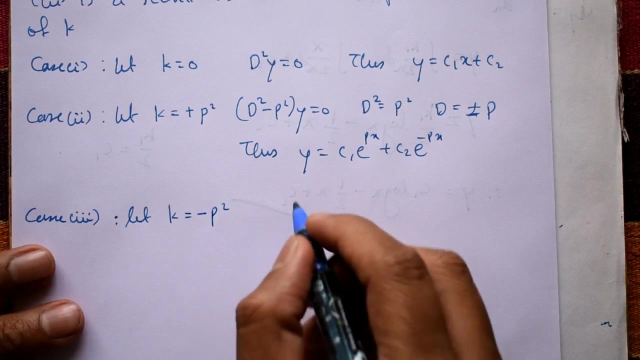 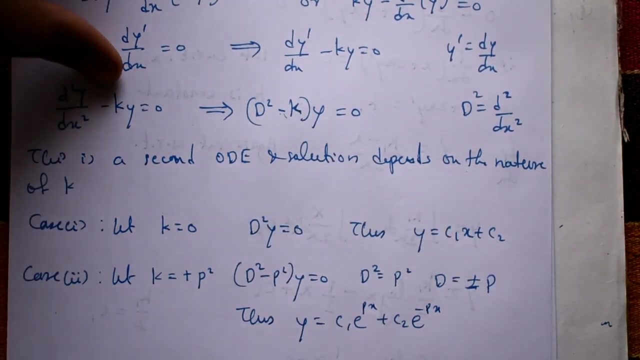 c1 e raise to px plus c2 e raise to minus px. okay, now third case. and k is negative. that k is a less than 0 means k is equal to minus p square negative value. now take d square minus sign, d square minus k. k means minus p square, minus p square means: